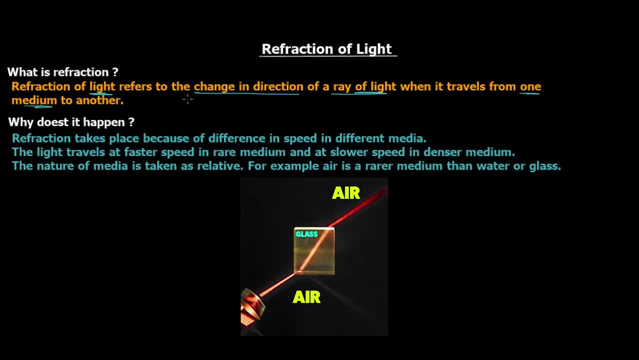 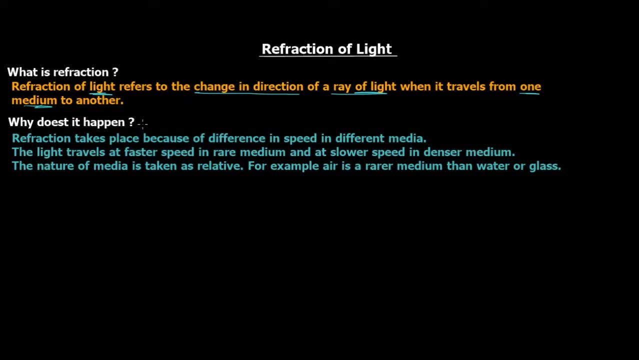 of the ray and again, when it exited the glass slab and entered the air, it was a slight shift in the air again. it again changed the direction. So this is the definition of refraction. So you must be wondering: why exactly does this happen? So that is question number two over here. Refraction takes 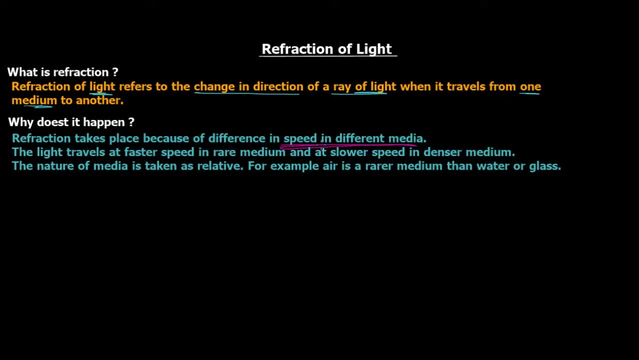 place because of difference in speed in different media. So this is the real reason why there is the shift of direction and refraction. So the light travels at faster speed in rarer medium and at slower speed in denser medium. Now the nature of media is taken as relative. For example, air is 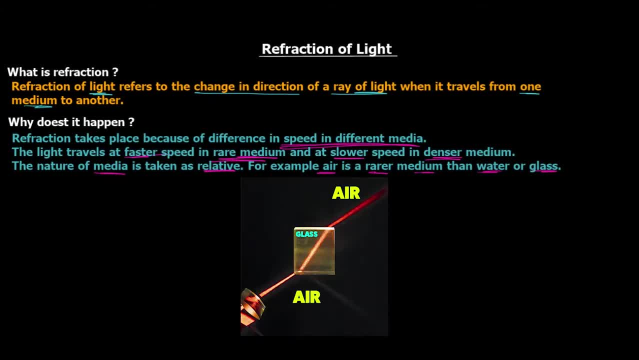 rarer medium than water or glass. So in the image where the laser first started to travel from the air, which was traveling in the air, it then entered the glass. Now glass, compared to air, is much more denser as a medium. So the speed of the laser when traveling through air is higher compared to the 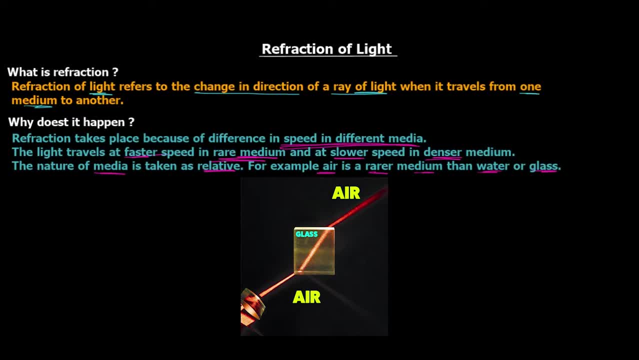 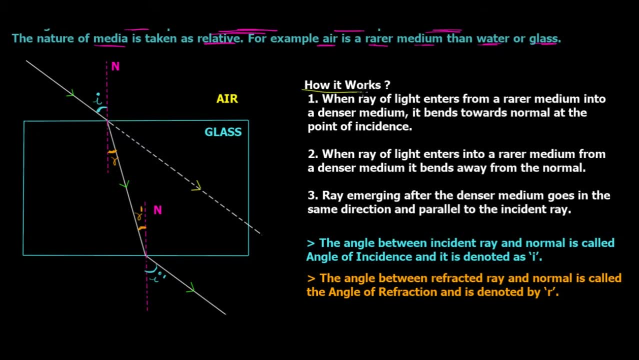 speed of the laser traveling through the glass. So this is what makes it change direction. So let's see how it works diagrammatically. Okay, so we have a diagram over here and we have three points. So the three points specify how refraction works. Now let me just first give you an overview of 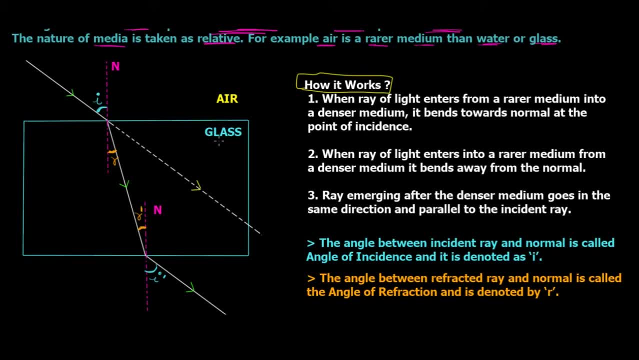 the diagram. So we have this blue rectangular box which essentially is a glass, So this is a glass medium. and then I have written air and this is a ray of light which is falling on this glass and it is meeting at this point. This pink dotted line is an imaginary line which is perpendicular to the 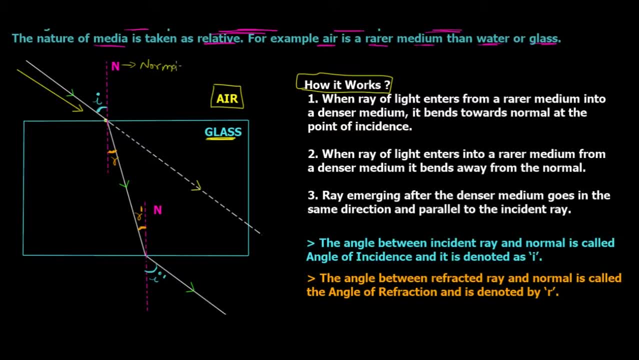 glass and it is known as a normal. So this is a normal, or we call it as a normal. So let me just read out the first point. When ray of light enters from a rarer medium into a denser medium, it bends towards the normal at the point of incidence. So this is a ray of light which is incident on the 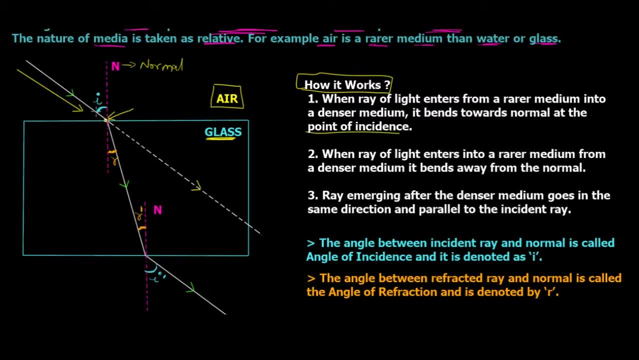 glass. So this is the point of incidence and it is making an angle of I with the normal. So this is known as the angle of incidence. that is, the angle between the incident ray and normal is called angle of incidence and is denoted by I. Now what they are. 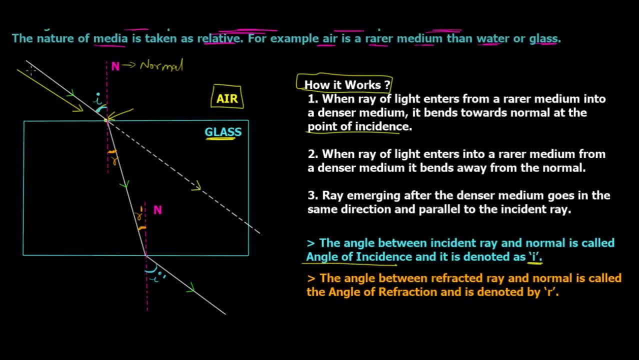 seeing is when a ray of light enters from a rarer medium. So since the ray is starting from air, it is in a rarer medium, that is, it is in a less denser medium, and it enters a medium which is denser than air. So it enters glass at this point. So what happens is it bends towards the normal. So you 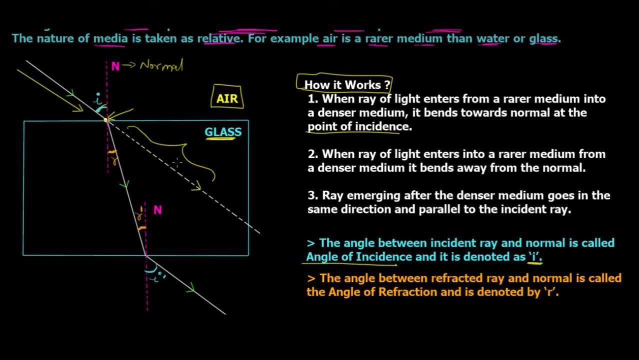 can see this dotted line. So this is how the ray of light should pass: in a straight line. but since the rarer medium is changed, it bends towards the normal and makes a new angle, which is known as the angle of refraction, which is denoted by R. So let's move on to point No.2 now. it says: when ray of 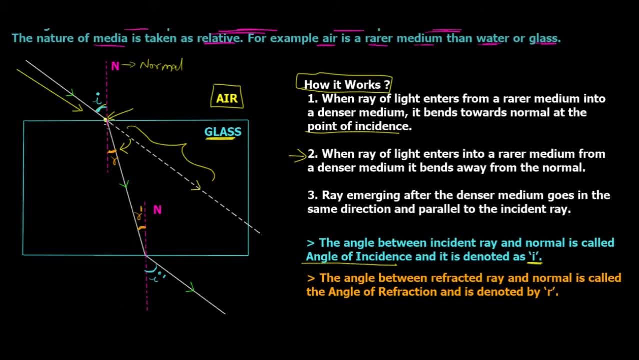 light enters into rarer medium from a denser medium it bends away from the normal. So now, once inside the glass, it again travels in a straight line. you can see over here like this. and once it exits the glass it moves away from the normal. So when it entered, it move close to the normal and this is. 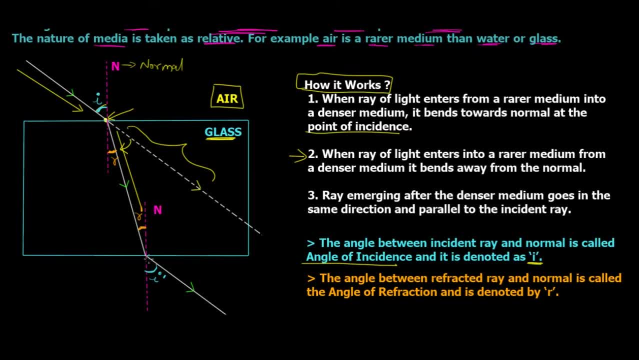 again one more dotted pink line, which is the normal again, which is perpendicular to the glass slab, clearly that it is moving away from the normal and it creates again one angle which is equivalent to the angle of incidence, which is represented by i dash, and this is again r dash, which is equivalent. 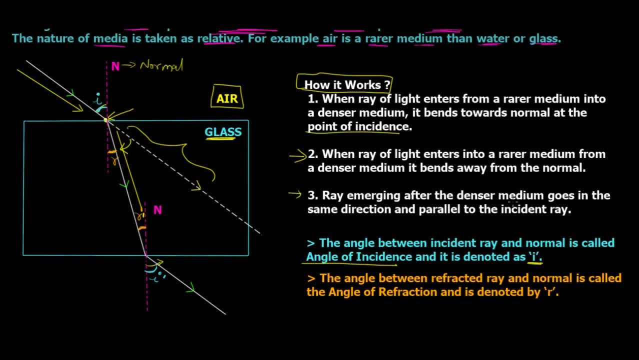 to angle of refraction. Now the third point says the ray emerging after the denser medium goes in the same direction and parallel to the incident ray. So this ray that is exiting is parallel to the ray that entered. So they will never meet, but they have slightly changed direction. Actually, the 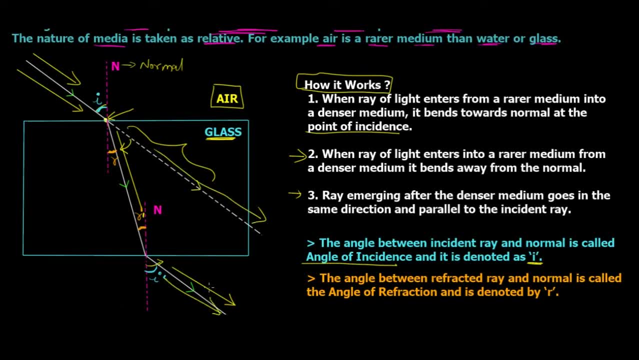 ray should be going like this, but it is going this way, in the same direction and in parallel, but it should be over here, but since the medium changed, it traversed from here. So this is how it works diagrammatically. Now let's see what refractive index is. So refractive index is the 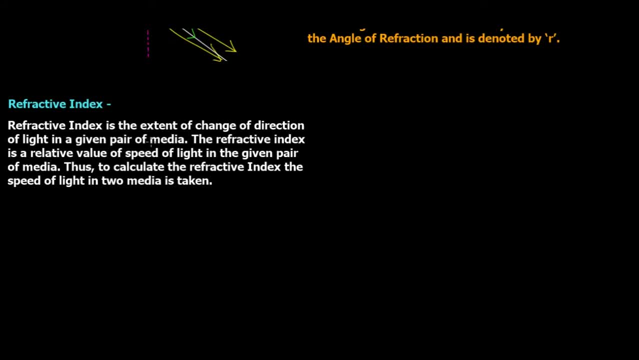 extent of change of direction of light in a given pair of media. So let me just read it out again: Refractive index is the extent of change of direction of light in a given pair of media. So the refractive index is relative value of speed of light in the given pair of media. Thus to 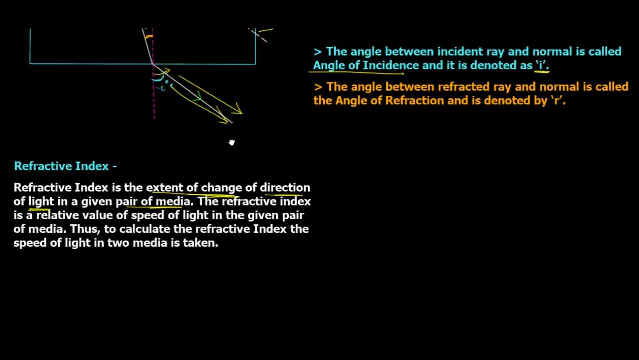 calculate refractive index. the speed of light in two media is taken. So by this definition the ray is going to be in the same direction as the light in the given pair of media. So this refractive index of glass with respect to air is going to be a constant value and the refractive 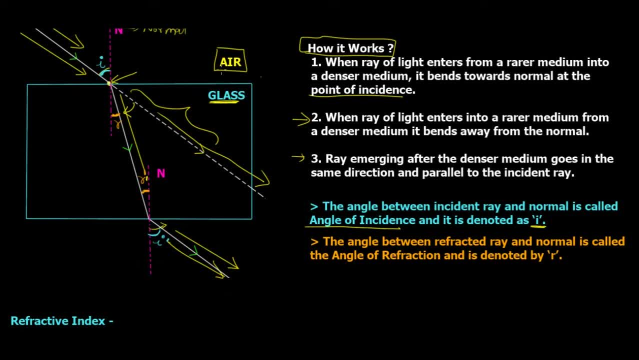 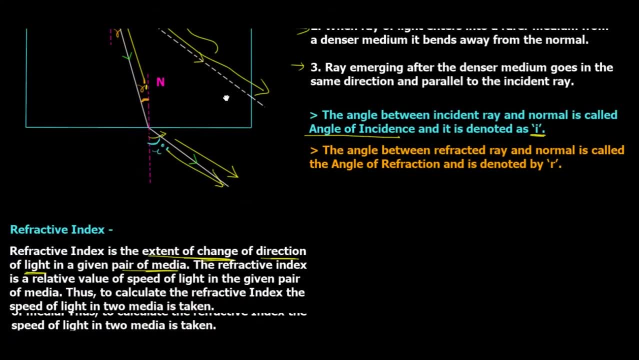 index of air with respect to glass is again going to be a constant value because, since the medium does not change, the extent to which the ray of light is going to divert or refract is always going to be same. So this is what the definition says. So now we have a formula to calculate this. 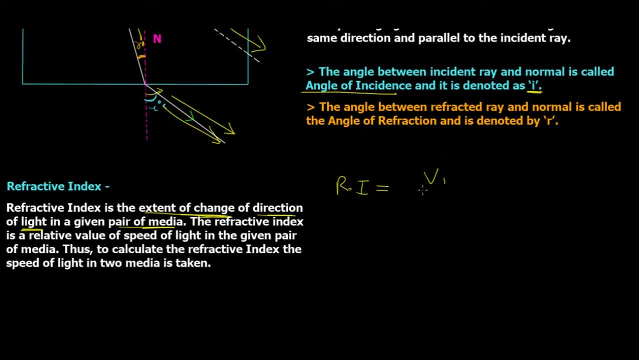 refractive index, let's say ri, and it is given by v1 upon v2.. So this v1 is speed of light in medium 1, which in this case is air, and v2 is speed of light in medium 2.. So this v1 is speed of light. 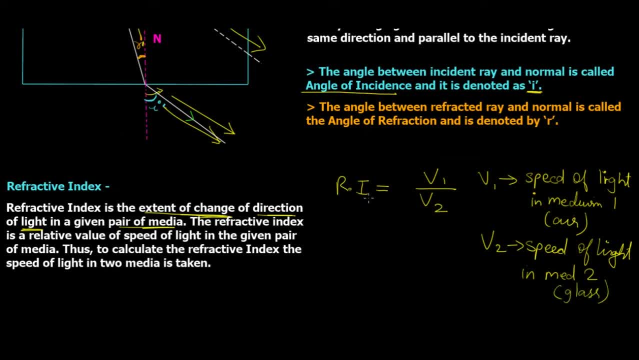 in medium 2, which is glass, So this refractive index is for medium 2.. So this refractive index is for glass. with respect to air, Similarly, refractive index of medium 1, which is air, would be v2 upon v1 and v2 would be speed of light in medium 2, that is glass, and v1 is speed of light. 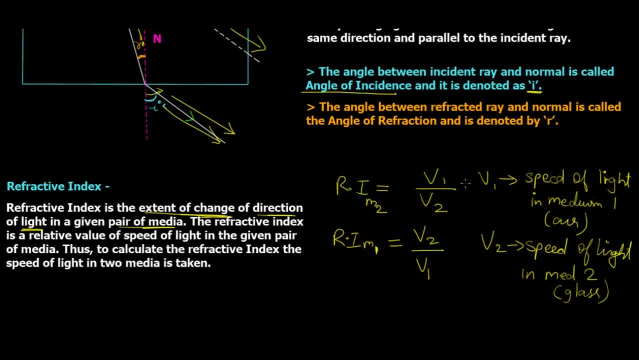 in medium 1.. So these values are always going to be constant for certain pairs, for example, air and oil, glass and water, air and water. So these combinations are always going to be constant for the refractive index for the particular pair of media. So this is what the definition says. 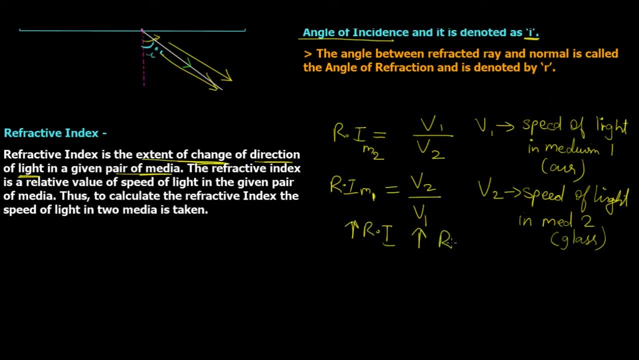 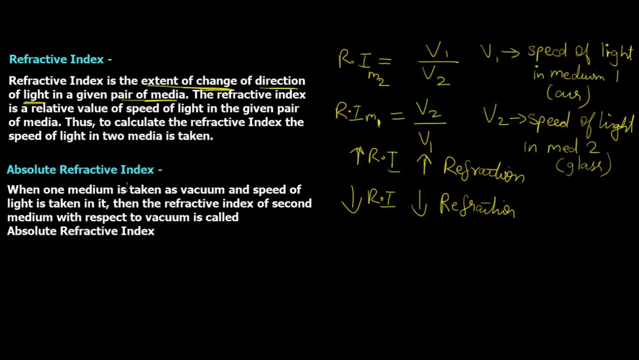 Also higher the value of refractive index, higher the refraction and lower the value of refractive index. lower the refraction. Now let's see one more concept of absolute refractive index. So the definition of absolute refractive index is when one medium is taken as vacuum and the speed 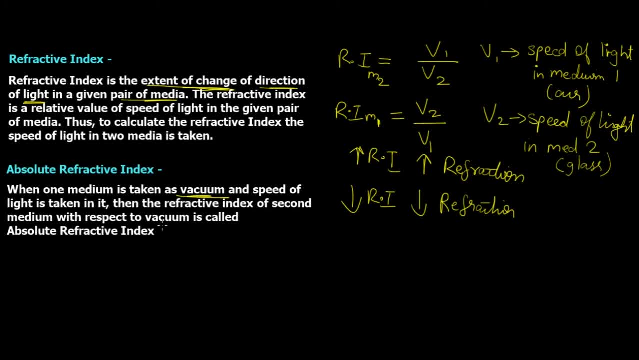 of light is taken in it. the refractive index of the second medium with respect to vacuum is called absolute refractive index. So in the speed of light in vacuum is the highest, which is 3 into 10, raised to 8 meter per second. So whenever we calculate the speed of light in vacuum, 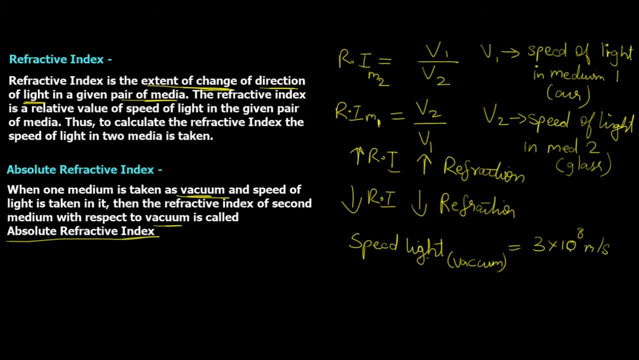 we are calculating the absolute refractive index of any medium with respect to speed of light in vacuum. At that time we are calculating the absolute refractive index of that medium. So in that case, Ri of glass with respect to vacuum would be speed of light in vacuum upon speed of light. 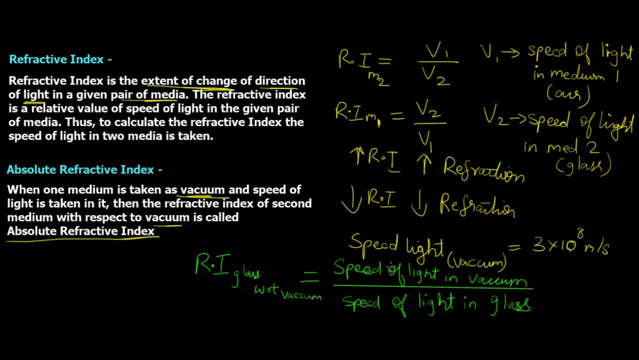 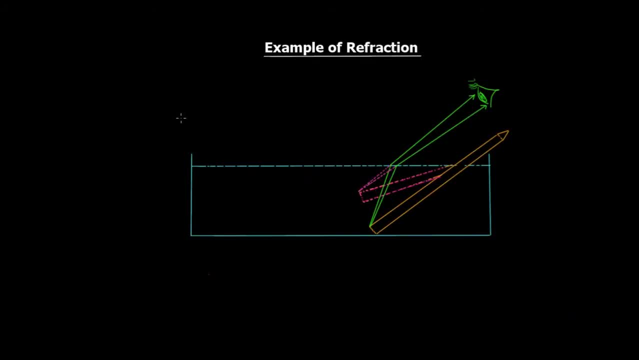 in glass, or refractive index of air with respect to vacuum would be speed of light in vacuum upon speed of light in air. So that's how we get the absolute refractive index. Okay, so these were the some basic concepts of refraction and how it works. Thank you for watching this video. If you liked it. 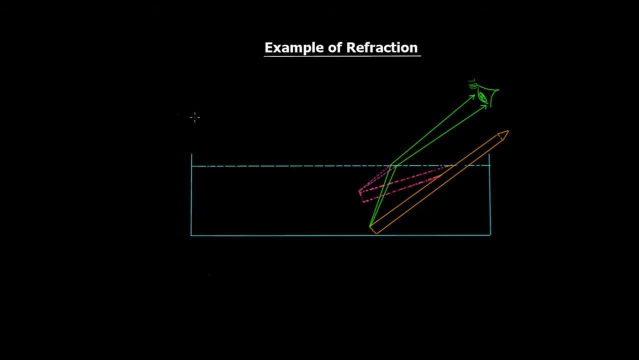 don't forget to subscribe to my channel and hit the bell icon so that you don't miss any of my new videos. So now let's go back to the earlier example, which was a real world example, as in: why do objects inserted in water appear closer than they actually are? So here's a diagram which I've drawn So you